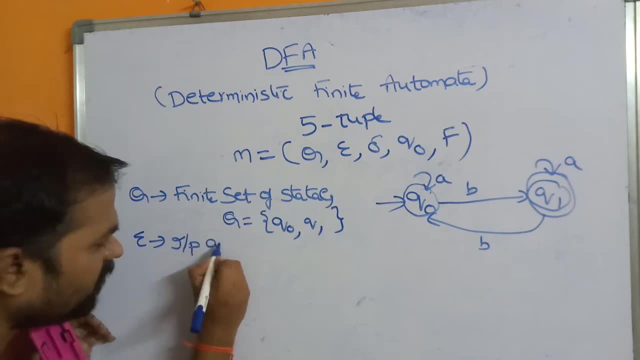 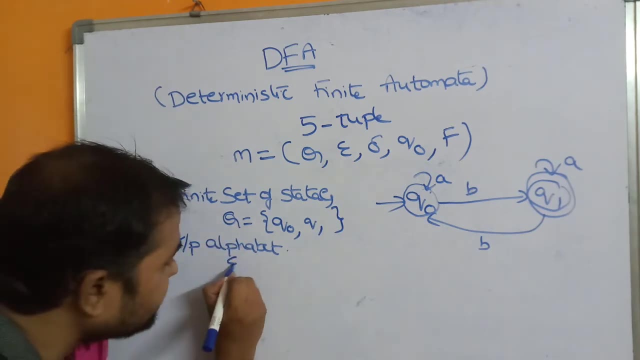 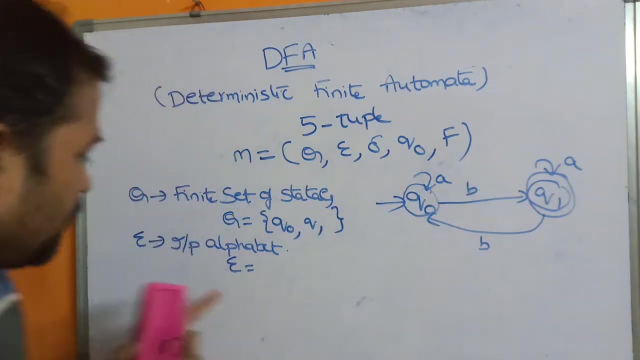 nothing but input alpha bit. So we know what is alpha bit. Alpha bit means a set of symbols, a set of symbols. So what are the symbols in this diagram? Here we have two symbols. The first symbol is A, the second symbol is B. So here the alpha bit contains: 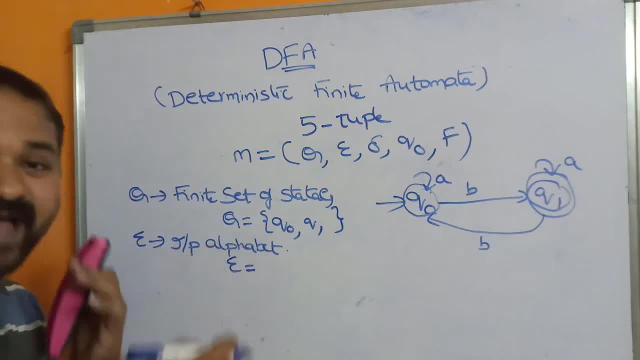 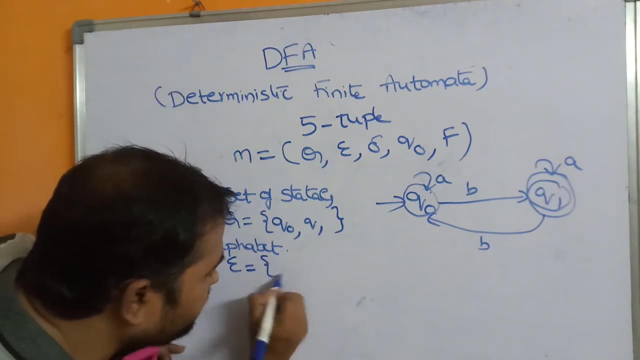 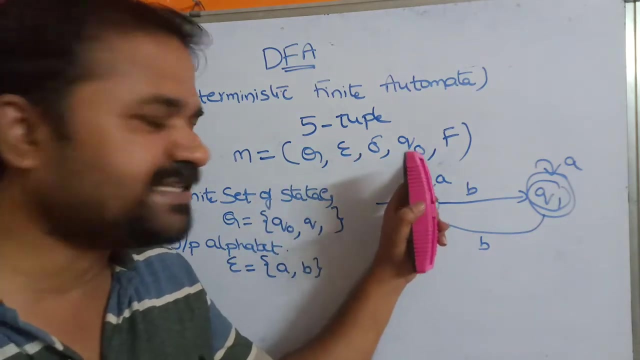 two symbols. So that is why here I am saying that sigma means an input, alpha bit, set, set of symbols. So set means the collection of symbols. So we have to use this: curly braces. So A, comma, B. Now let us see, we will see. about delta ladder: Now let us see. 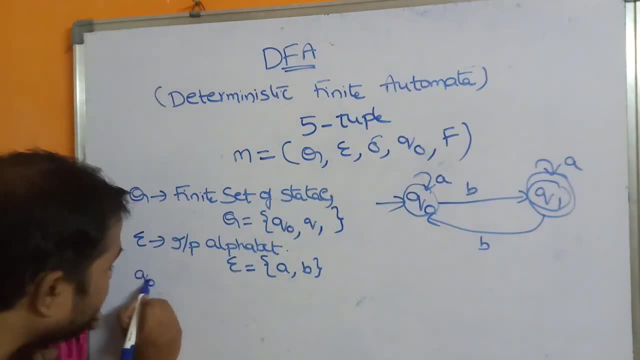 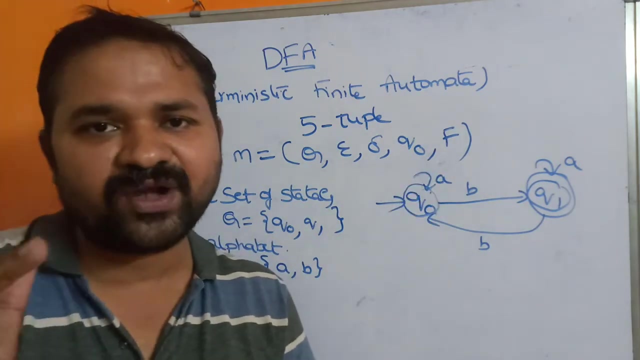 the next one: Q naught. What is Q naught? Q naught means initial state. Here in DFA, we can have in DFA or NFA, we can have only one initial state, one initial state. So there is no need of a set of initial states. So we can have only one initial state. So how? 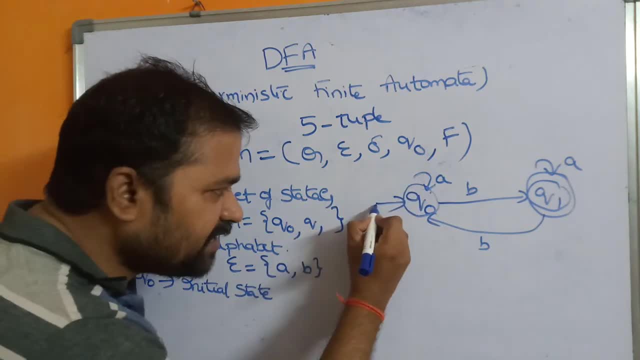 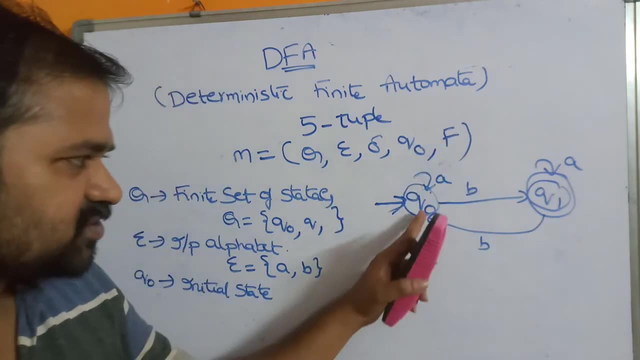 to represent initial state. So initial state means here we have a set of initial states, So we have to use this arrow like this, So arrow and after that, within the circle, we will represent the initial state. So what is the initial state present in this diagram? 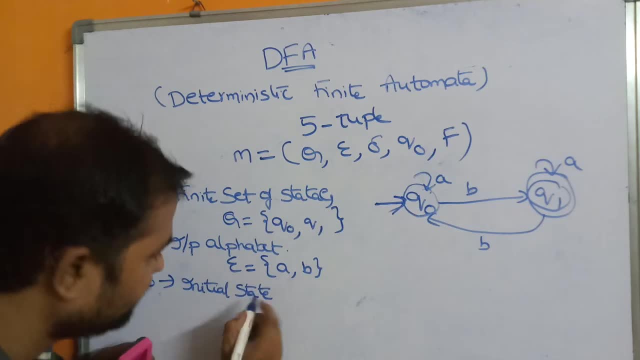 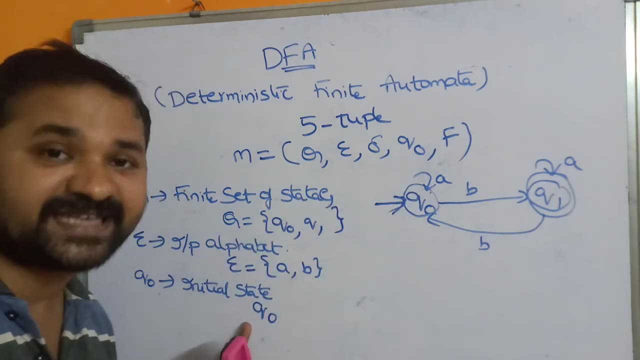 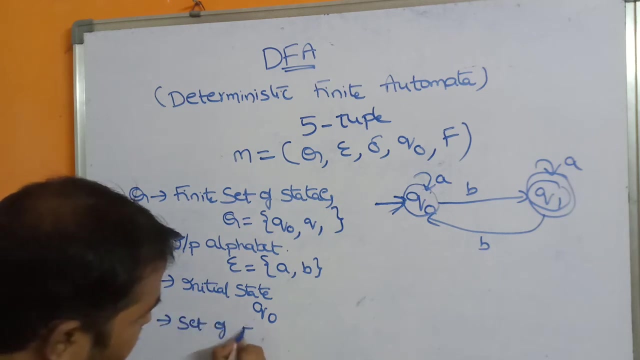 Q naught. Q naught Why? Because here we have arrow, is there? So Q naught is the initial state, So there is only one initial state for the mission, So there is no need of any set here. Now let us see about what is F. F means a set of final states, F means a set. 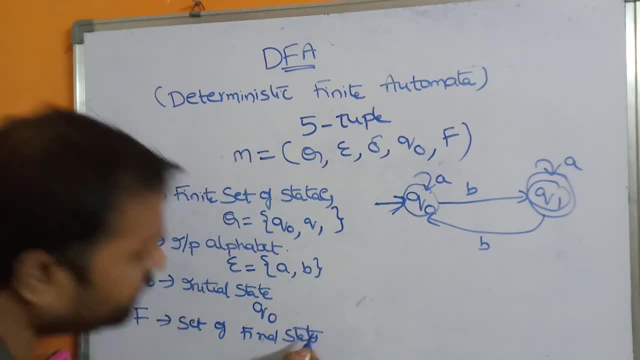 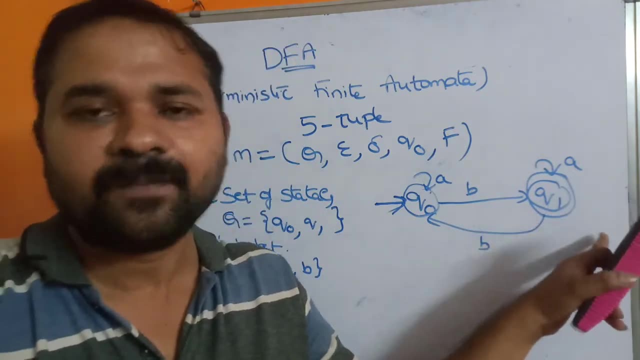 of final states. So that is the initial state. Now let us see about what is F. F means a set of final states. That means here our mission may contains more than one final state also, But here we have only one final state only, But we can have multiple final states. 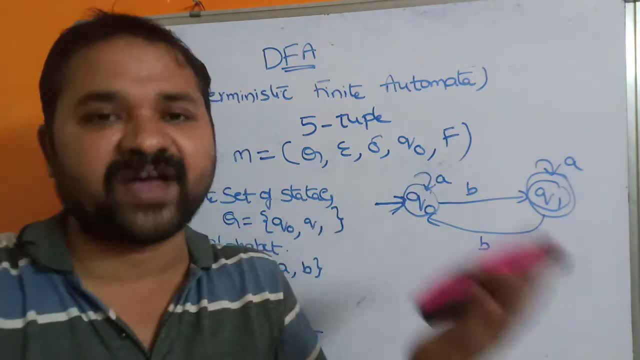 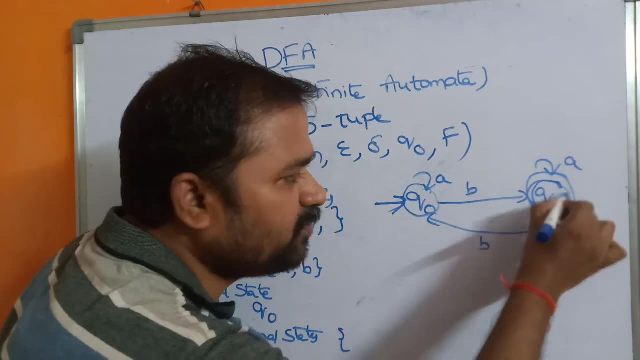 also. But this is a set. We may have multiple final states. So that is why we have to use this curly braces. Within the curly braces final state means we have to use the double circle. So within the double circles we have to place the state name. So here what? 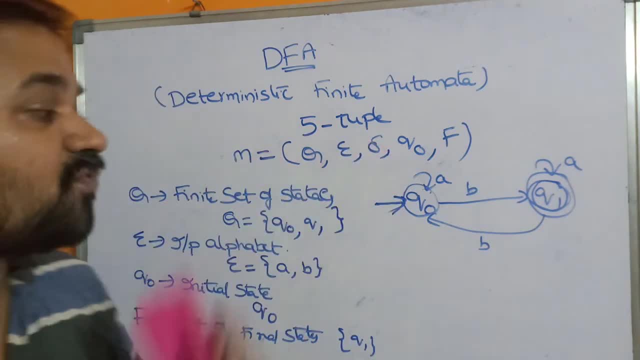 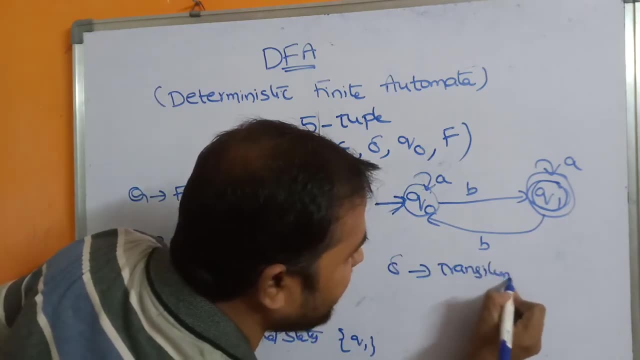 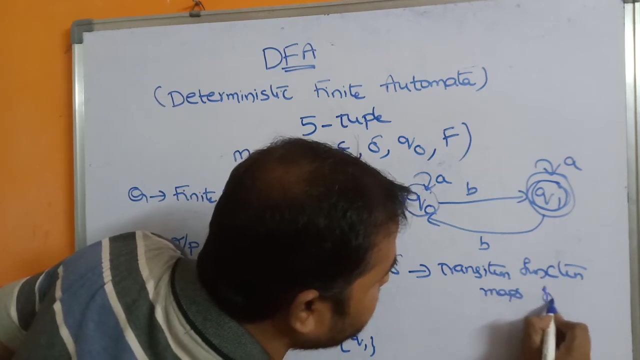 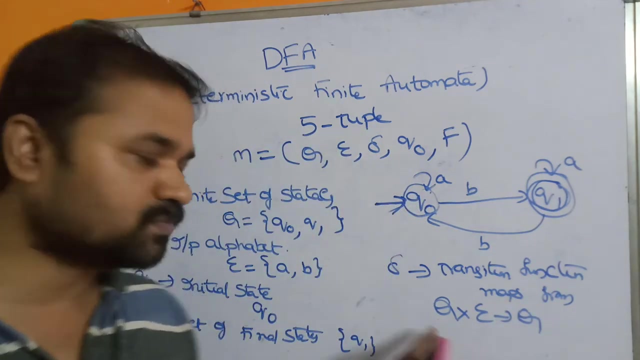 is the final state. Q1 is the final state. Now let us see about what is F. F means a delta. Delta is a transition function. Delta is a transition function which maps from Q cross sigma to Q, Q cross sigma to Q. So here, what is Q? Q means a set of final state. 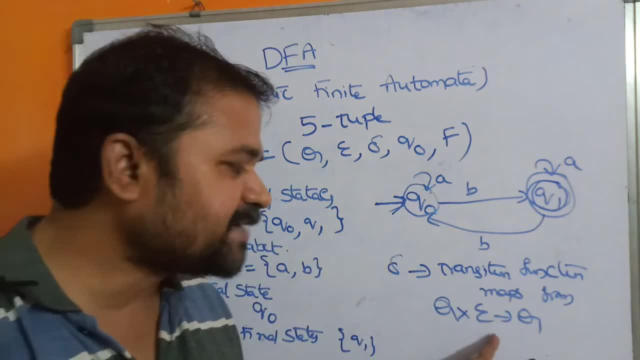 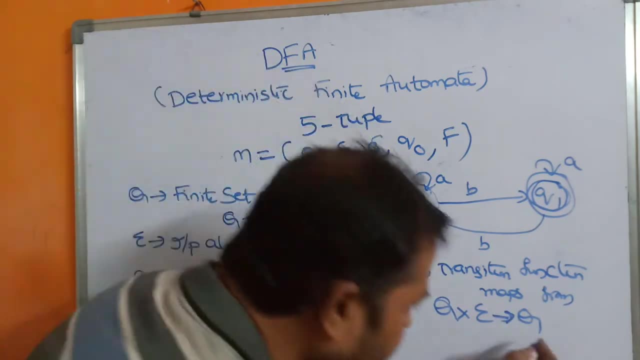 So it may be any state. It may be either Q naught or Q1.. Sigma means input alphabet. This is nothing. This is nothing but transition. So this is nothing but Q. So it is generating Q. So 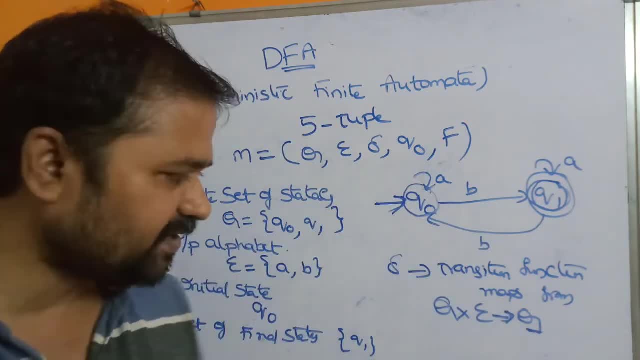 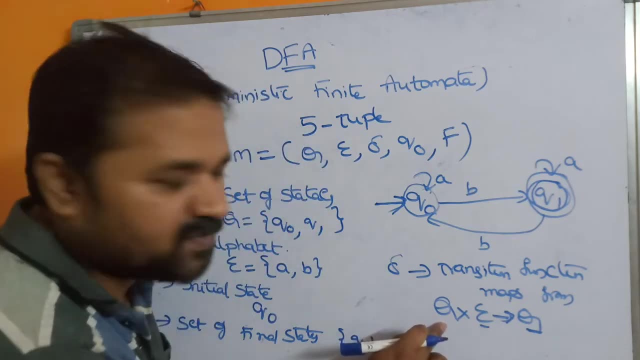 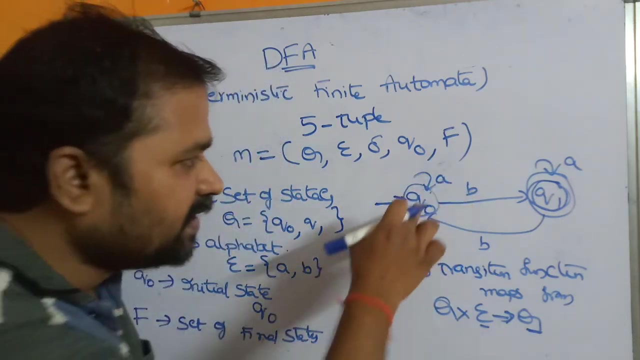 what is Q? Q is nothing but one of the state here. Let us see what is the mean here. If we apply an input symbol on one state, we can go to another state. Let us observe this diagram. What are the transition functions in this diagram? If we apply a on Q, naught. 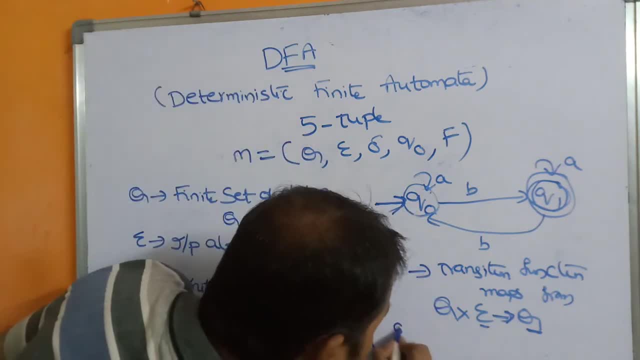 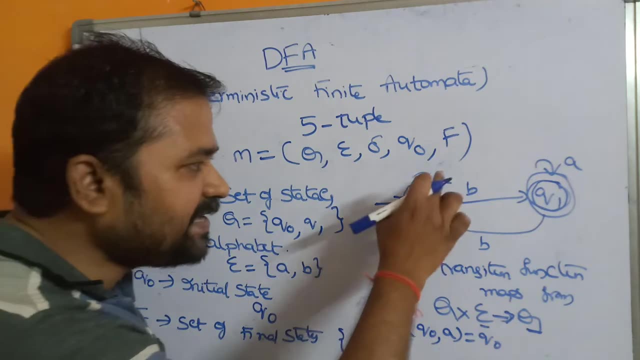 then we are moving to Q naught only. So here the first state. First transition function is delta of Q naught. comma a is equal to Q naught. So if we apply a on Q naught we are getting Q naught only. So this Q naught is nothing but this state. 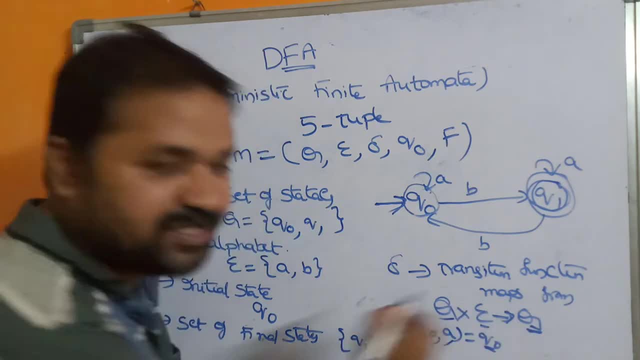 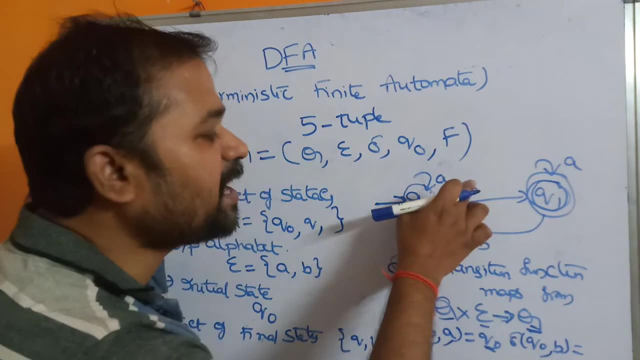 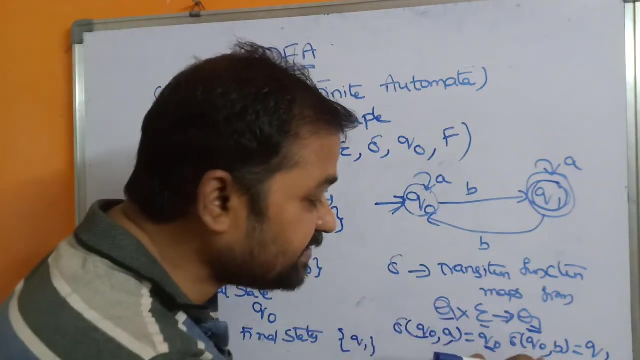 This sigma is nothing but a and this state is nothing but this Q. So like: what is the next transition function? Delta of Q naught, comma b is equal to. If we apply b on Q naught, we are moving to Q1 state, Q1 state. So this Q is nothing. 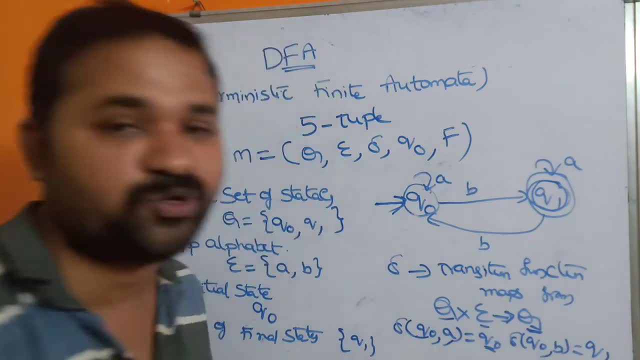 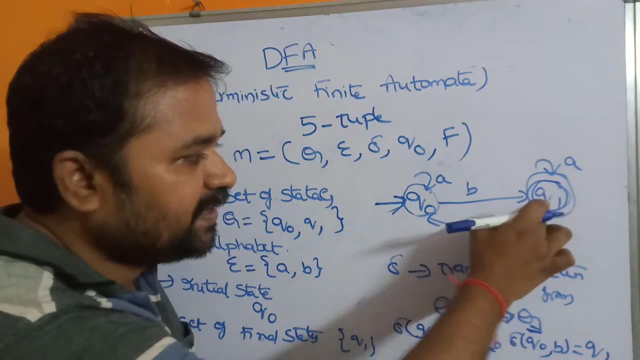 But Q naught Sigma is nothing but b. This Q is nothing but Q1.. So, likewise, if we apply a on Q1, then we are getting Q1. only If we apply b on Q1, then we are getting what Q? 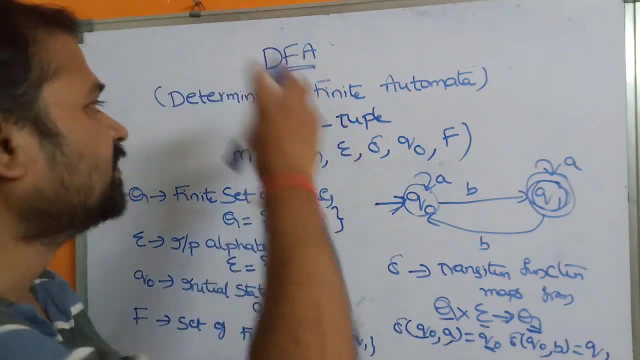 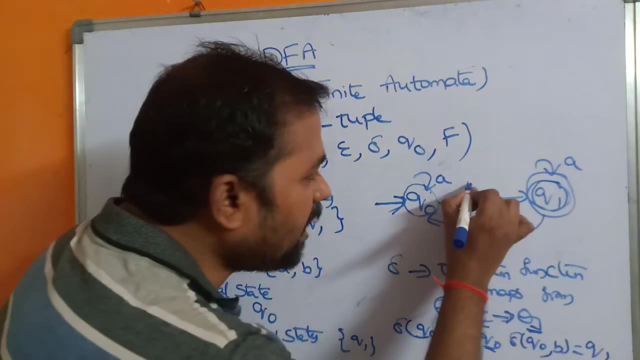 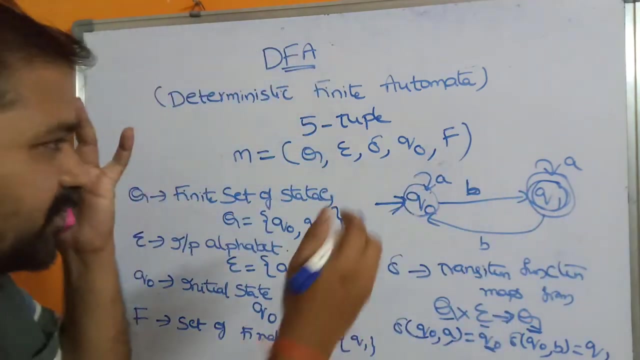 naught state. So in this way we can define d of a. Why it is called as deterministic finite automata? Why? Because if we apply an input symbol on a state, then we can define only one state. So if we apply an input symbol on a state, then we can get only one state. 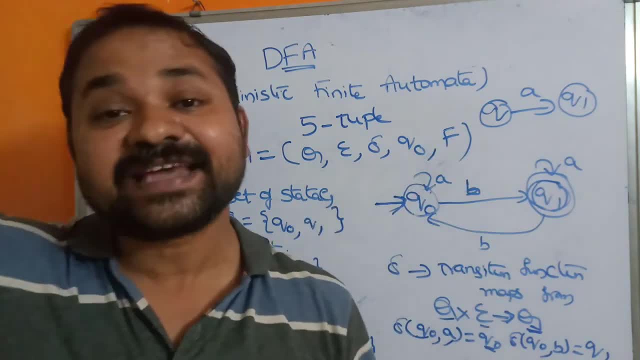 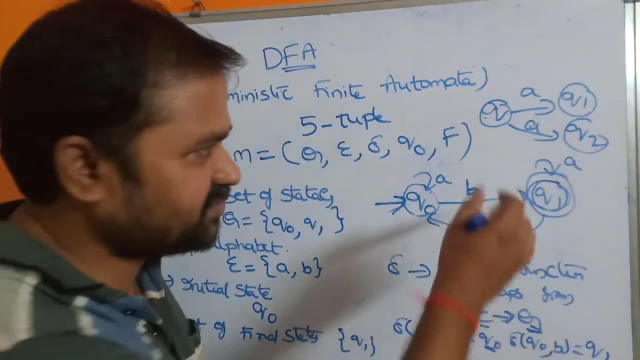 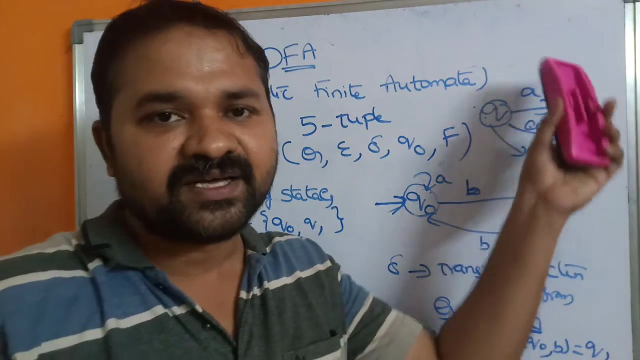 So that is why it is called as d of a, Whereas in NFA if we apply a particular input symbol on a state, we can get multiple states. So here we are applying a only on Q, but we are getting different states: Q1, Q2, Q3.. So that is why this is called as NFA. 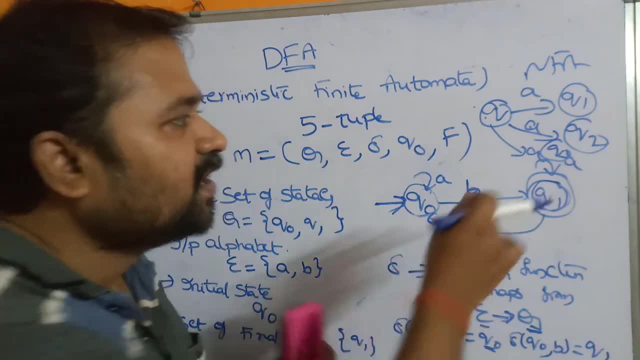 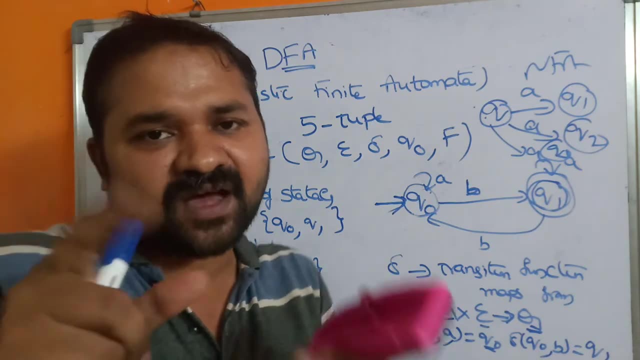 We will see this in the next video. Whereas d of a means if we apply an input symbol on a particular state, then we can get only one state. So that means on a particular input symbol for a particular state, there will be only one edge, There will be only.